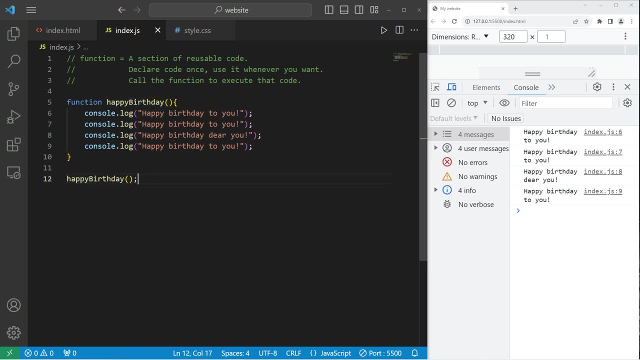 you type the function name, then you add a set of parentheses. I like to think of the parentheses as two telephones talking to each other. That's how I remember it. So if I were to call this function again, what do you think is going to happen? Well, we're going to execute this function. 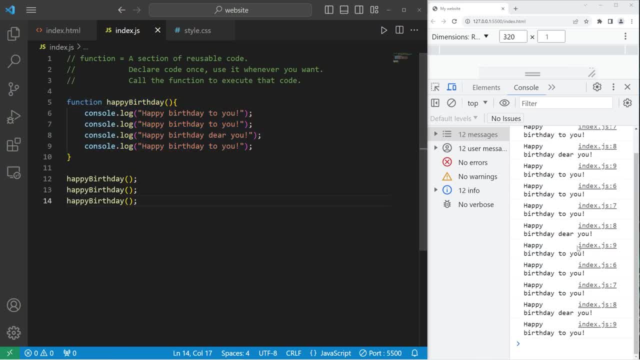 twice, Three times. We'll execute it three times As many times as I want. in fact, That's what a function is. It's a section of reusable code. Reuse it whenever you want. You just have to call it. You can send a function, some values or variables. Let's change our happy birthday. 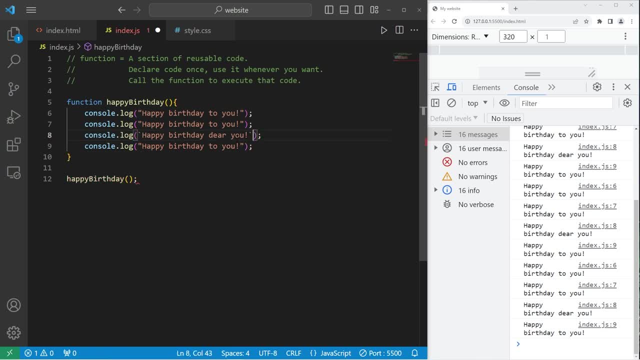 function. I will turn this line into a template literal. Let's replace you with the placeholder, Then we'll add a username. I'll add one more line. We'll use a template literal. You are a placeholder- Age ears old. So when I run this program we have an uncaught reference error. 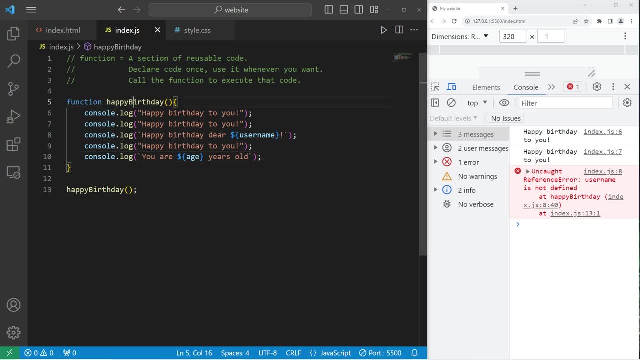 Username is not defined at happy birthday, So our happy birthday function doesn't know what our username is or the age, So we can send some information to the function when we call it. So, within the set of parentheses, what would we like to send this function? Let's send our name. 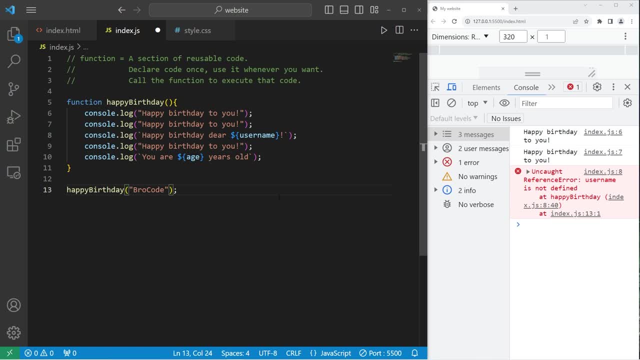 So whatever values you place within the function, be sure to comma separate them. So why don't you go ahead and send the happy birthday function- a name and an age- But there's one step missing. These are known as arguments. They're data that you send a function, But you 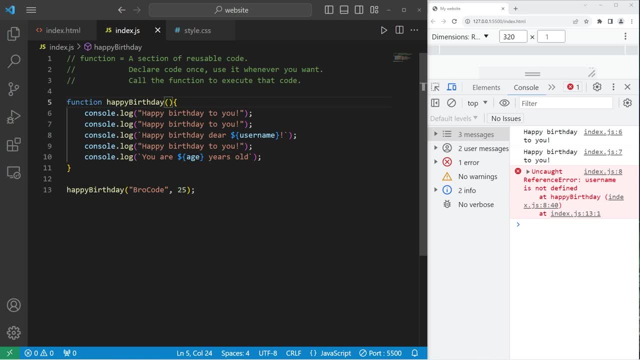 need a matching set of parameters Within the parentheses of the declaration. in a way, we can define some temporary variables And they're all comma separated, So let's go ahead and send a separated. We will define a username parameter as well as age. Now this function should work. 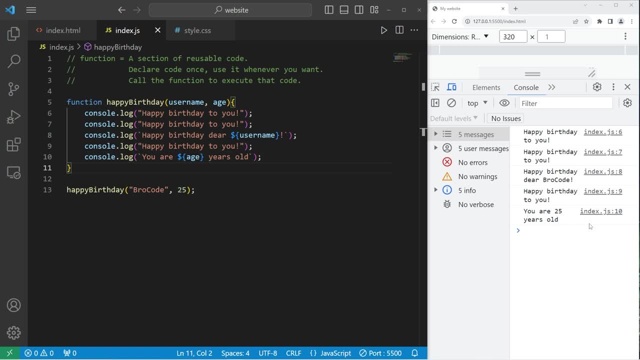 properly. Happy birthday, dear bro code. you are 25 years old, So these are parameters and what you send, the function, are arguments. Let's call the function, but send different information. Happy birthday. How about Spongebob? Spongebob will be. I don't know how old he is. according to Spongebob lore, but let's say he's 30 years old. Happy birthday, dear Spongebob. you are 30 years old. How about Patrick? this time It's his birthday. Everybody gets a birthday. Patrick will be 37.. Happy birthday, dear Patrick. you are 37 years old. So that's a benefit of. 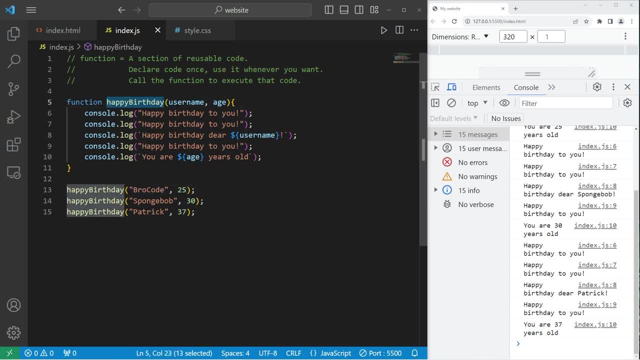 passing arguments to a function. When the function receives this data, it can do something with it. So let's say, I want to send a message to Patrick and I want to send a message to him Now. the order of the parameters does matter If I were to switch age and username. 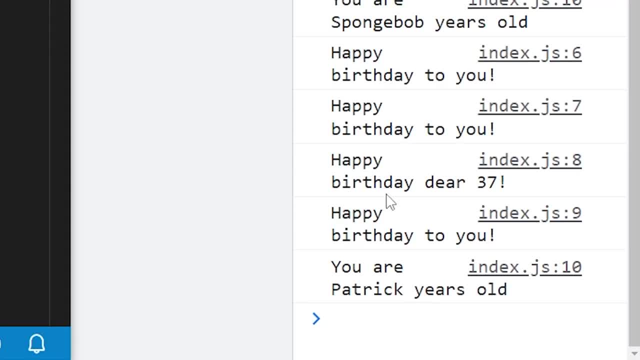 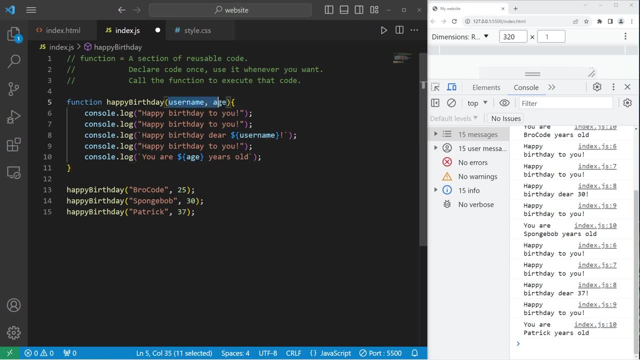 here's what happens. Happy birthday, dear 37,. you are Patrick years old. With the arguments that you're passing to your function, you'll want to be sure that the parameters match up. All right, now I'm going to cover the return keyword. We'll create a few other function. 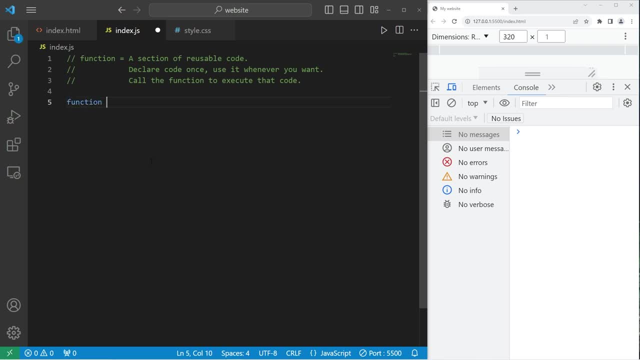 examples: We'll create a function to add two numbers- Function add. Then we'll need two arguments, which we will name x and y. So when we invoke this function, I would like to add x and y together. I'll create a temporary variable named result. 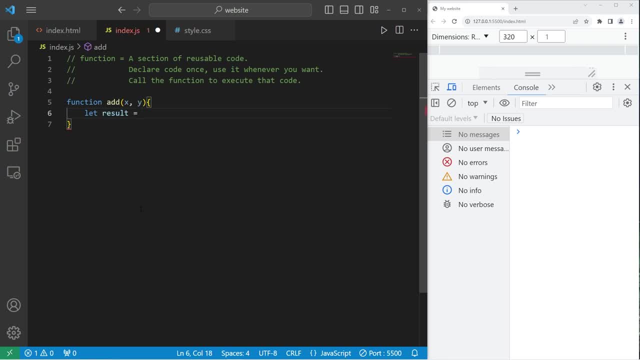 just to store the result. Result equals x plus y. So I'm going to add two numbers together. Let's add two and three together and let's see what happens. Well, nothing appears to happen. Well, we can send some data back to the place in which we call a function. 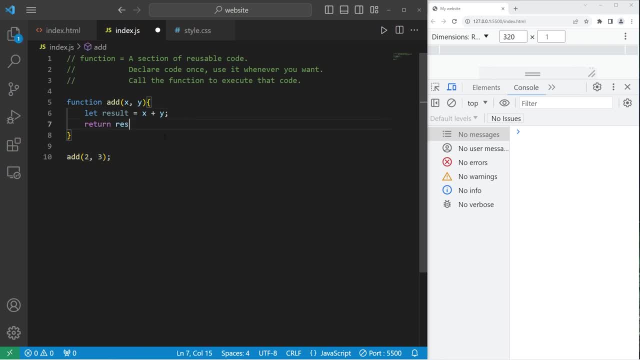 but we need to use this return keyword. Let's return the result. So two plus three should be five After this function resolves. think of this function becoming the value five. So we'll probably want to do something with that value. I'll store that within a variable. Let answer. 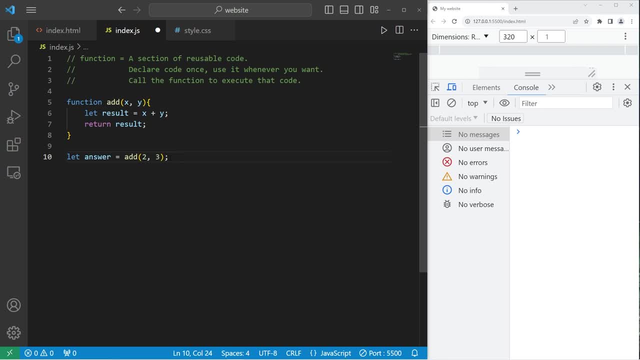 equal. add two and three, Then let's consolelog the answer, which should be five. When you return something from a function after you resolve the function, think of it as becoming whatever is returned. In this case, it's our result Or otherwise. I can place this function within consolelog. 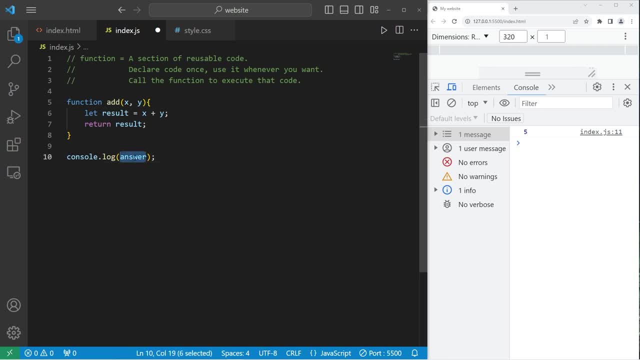 if we don't plan to store it at all. So add two and three, then display the result, which is five. There is a shortcut too. You don't necessarily need to declare a variable within this function. We could shorten this to return x plus y. That is also valid, So that should return five. 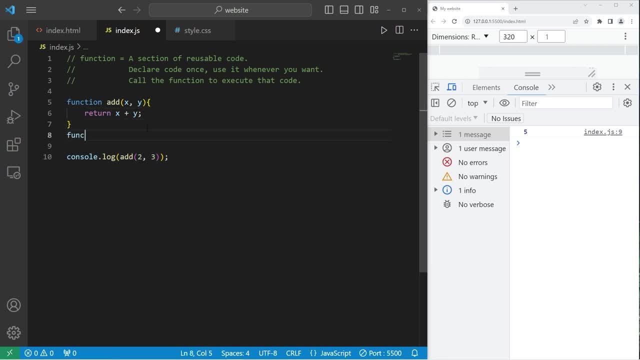 Okay, let's create a subtract function. Function subtract will return x minus y, but we need a matching set of parameters, because I forgot that. Okay, let's see what happens when we subtract three from two. That'll give us negative one. 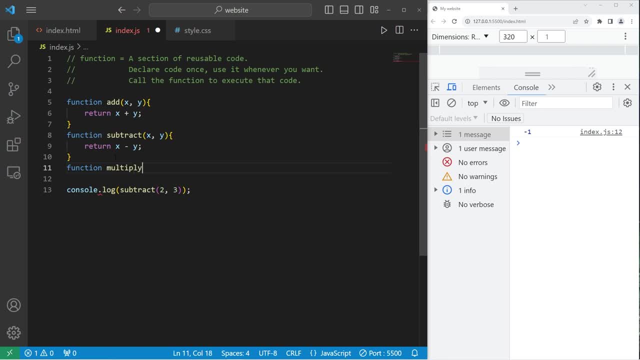 Let's multiply. Function Multiply. We'll multiply x and y together. Return x times y. We will multiply two times 3, which is six Divide. We need parameters x and y. And there we got two. Let's multiply it. Then we need a matching set of. 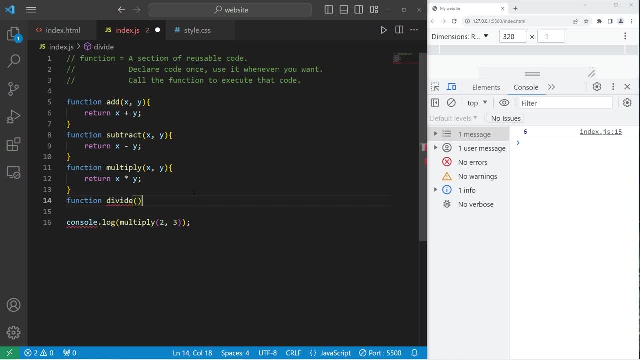 We need a matching set of mi. So we need a matching set of mi by the y. Let's say we get two TOP matrix category here Let me write trash cart. Let's figure out the ran to var metaphese. We're going to cost total Divide. We need parameters x and y. We'll get two x from below here, Sonra, and we'll have those. Then we'll make another option for our proof layer and that will give us our result. So to endpointgeb. 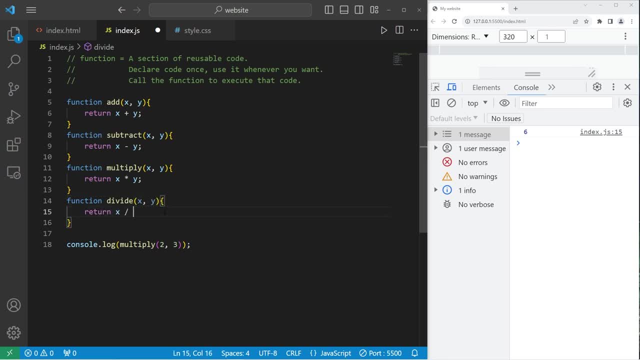 Send y, Then return x divided by y. Then we will invoke the divide function, Pass in 2 and 3. And the result is 0.666- repeating. Let's go over a more complex example. We'll create a function to determine if a number is even or odd. 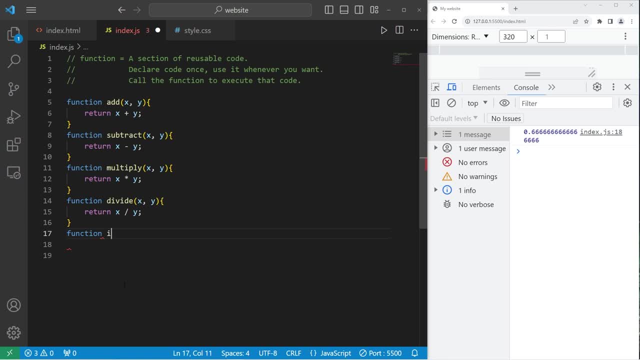 Here's the function. Function is even. We have one parameter, A number. So when we invoke the function, we'll have to pass in a number. So when we receive a number, how do we check to see if this number is even? 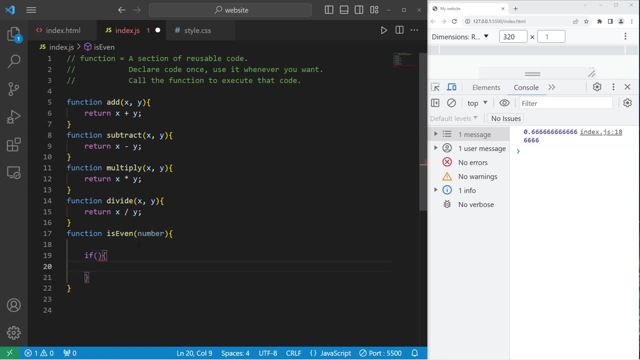 Here's one solution. We'll use an if statement. If our number modulus 2.. Modulus gives you the remainder of any division If this number divides by 2. evenly, if this is equal to 0, and yes, I'm using the strict. 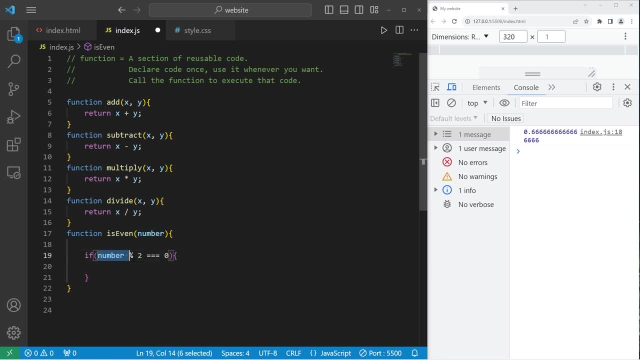 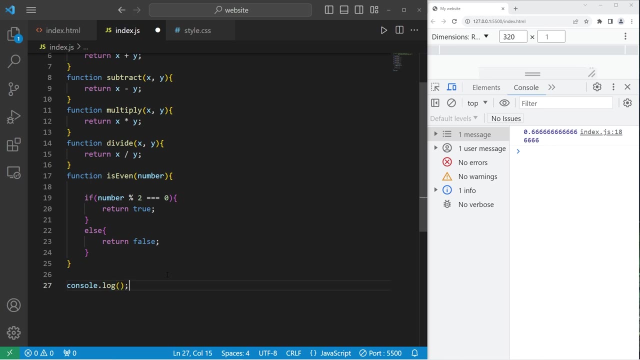 equality operator. I'm trying to use that more often. If our number is divisible by 2, then let's return the boolean value true, Else we'll return false. Okay, Let's consolelog. Let's check to see if a number is even. 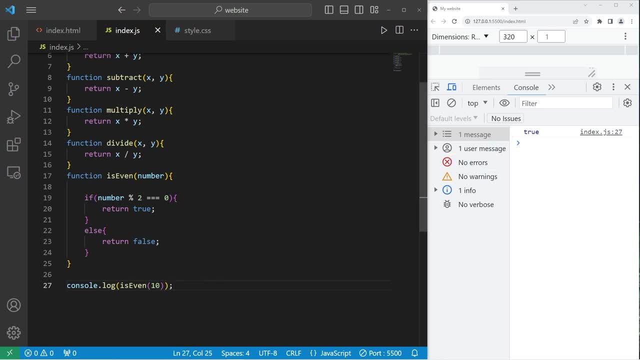 Let's start with 10.. Is 10 even? That is true. How about 11?? That is false. 12?- 12 is even. So that's kind of cool. If you would like a shortcut for this, you can use the ternary operator. 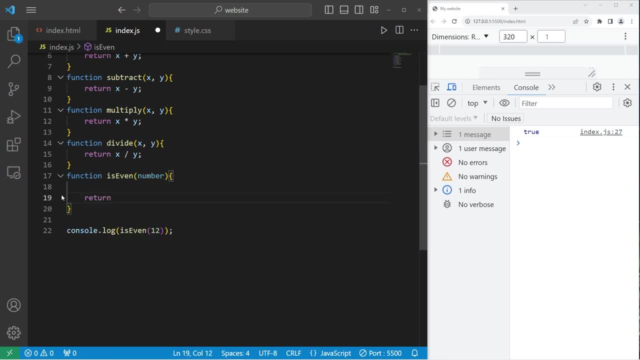 That would look something like this: We are going to return then a condition: What are we checking? Is our number modulus 2 strictly equal to 0?? So that is the ternary operator, the question mark. If it is true, then we will return a boolean value of true. 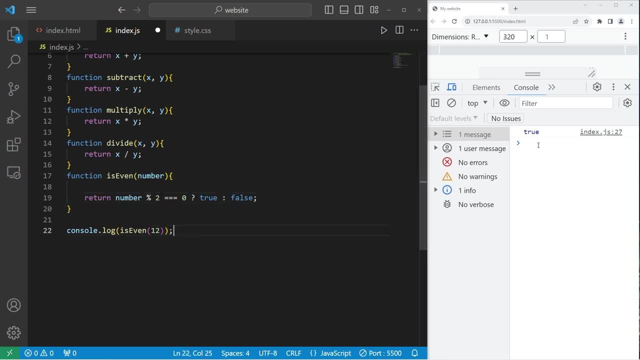 If it is false, then we will return a boolean value of false. Is 12, even. That is true. Is 13 even? No, it's not, It's odd. How about 14?? That is true, All right. 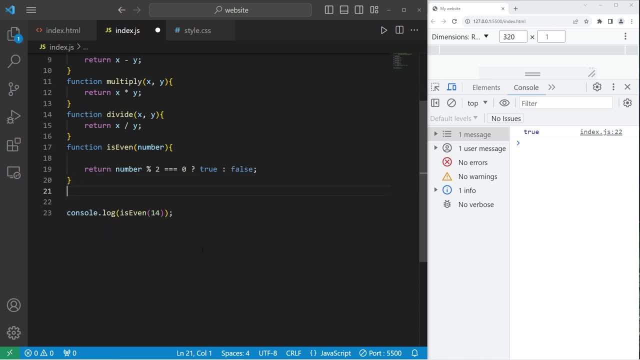 Last example. I think we're probably getting the hang of this now. We'll create a function to see if an email is valid. Function isValidEmail. What kind of information are we going to send? We'll set that up as a parameter. 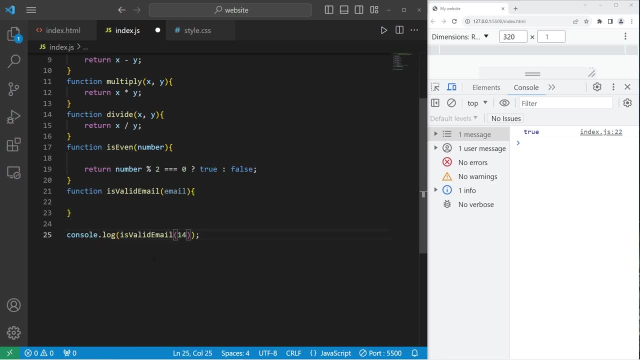 We will need an email. We'll invoke the isValidEmail function And pass in an email. Why don't you type in your email? I'll just make one up, Bro at fakecom. So when we invoke this function, this string of text will become our email. 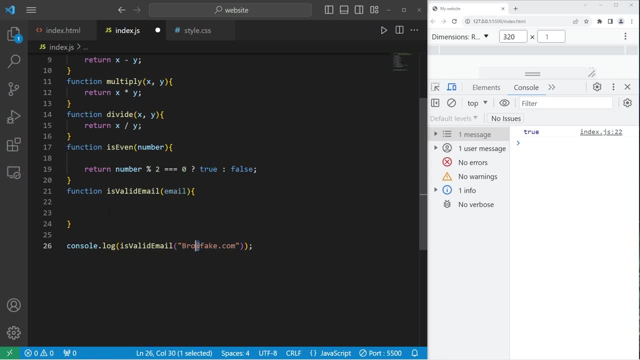 We'll check to see if our email contains the at character. We'll use an if statement If Email And there's a built-in method for this, The includes method. If our email includes the at character, then we will return true. 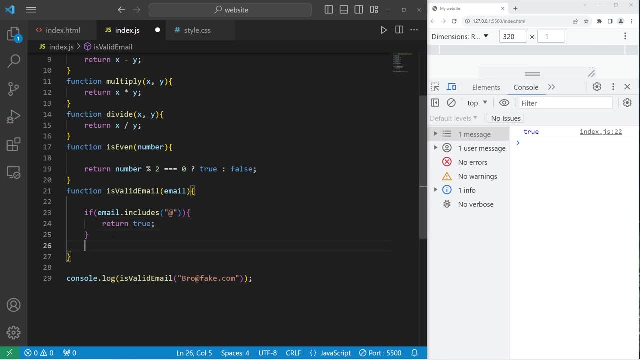 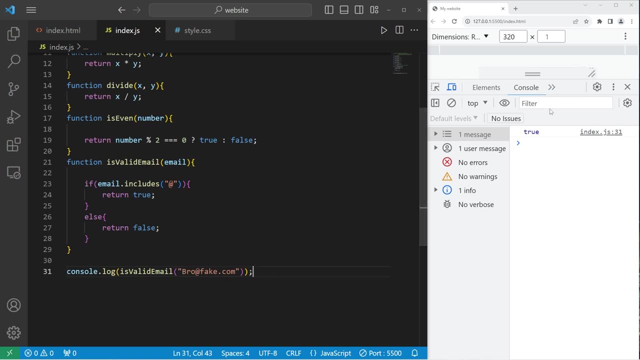 That is a valid email. They have the at character Else. we will return false. Is my email valid? That is true. Let's remove the at character Brofakecom. Maybe it's a website or something That is false. Let's try another email.